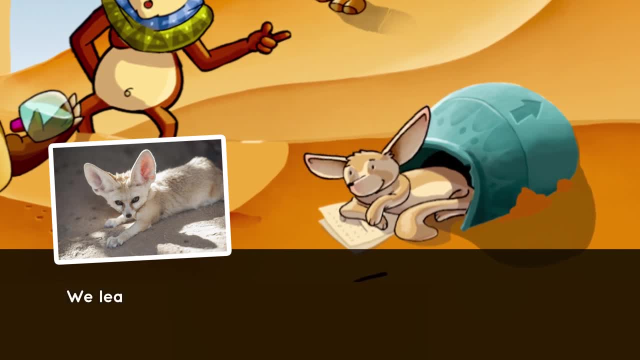 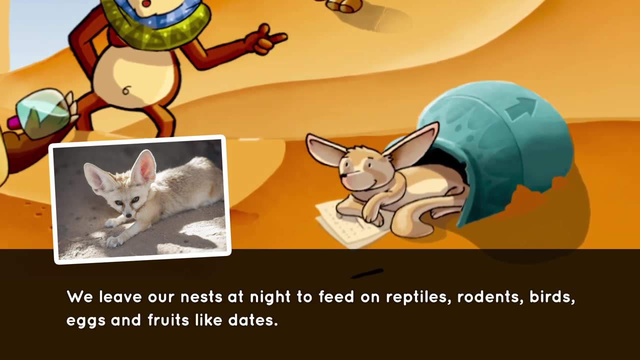 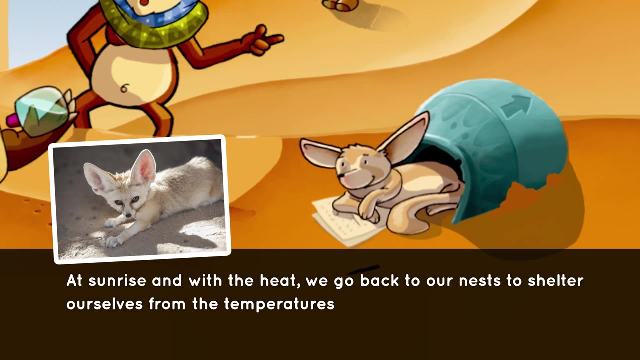 you know we're in October. You're right, We have only been in October for a few months. We leave our nests at night to feed on reptiles, rodents, birds, eggs and fruits like dates. At sunrise and with the heat, we go back to our nests to shelter ourselves from the temperature. 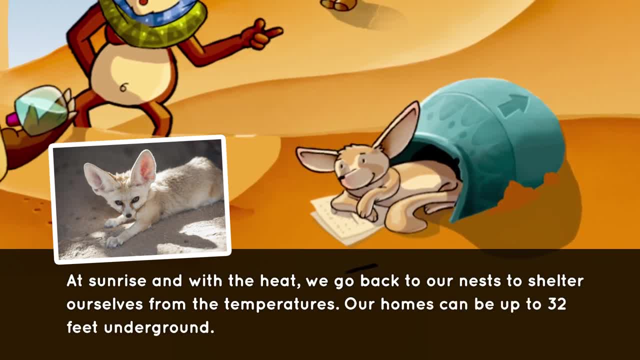 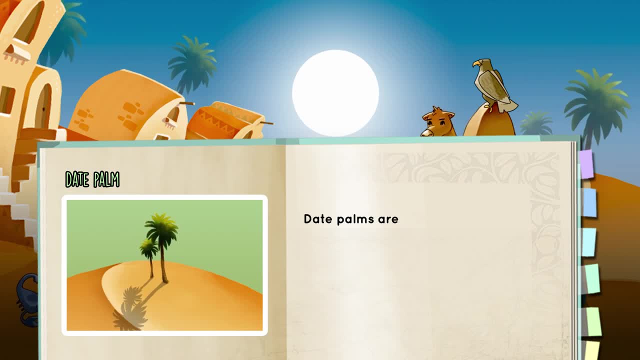 Our homes can be up to 32 feet underground. Date palms are our fruit tree, Our fruit. the date is the fruit of nature. It's the fruit of nature. It's the fruit can be harvested until the end of October. We live in very hot parts of the world that receive many hours of sunlight. 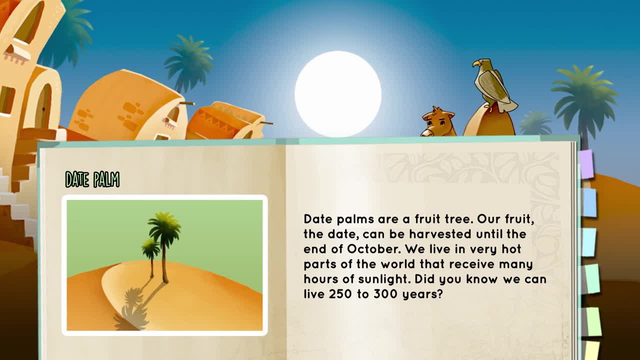 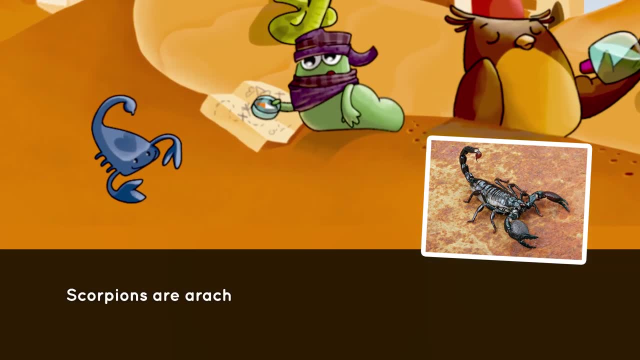 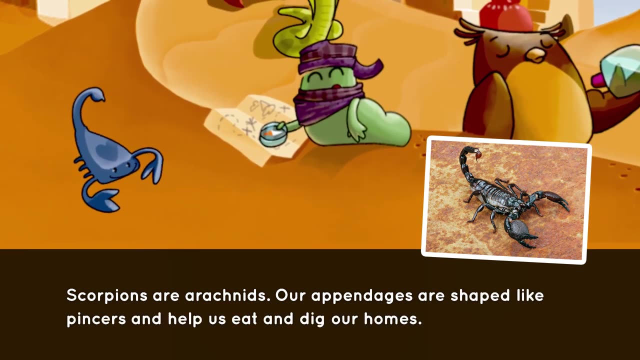 Do you know? we can live 250 to 300 years. Scorpions are arachnids. Our appendages are shaped like pincers and help us eat and dig our homes. Our tails end in stingers that contain powerful venom. 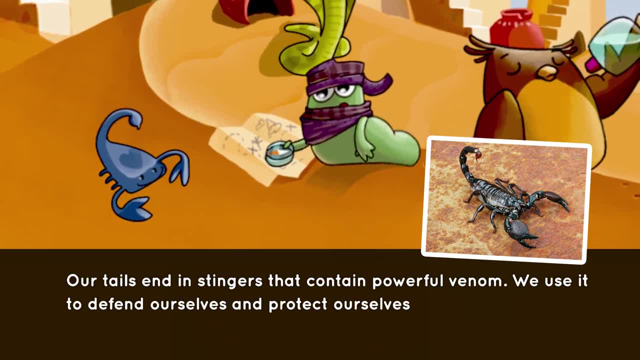 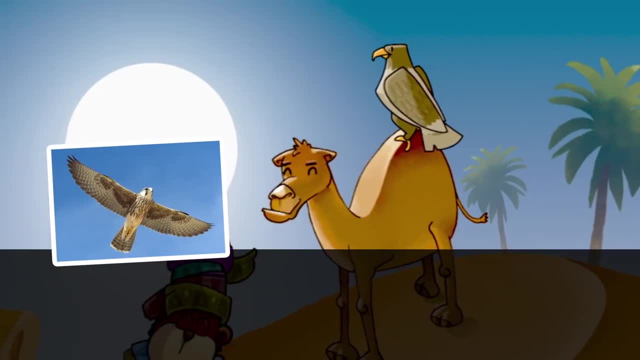 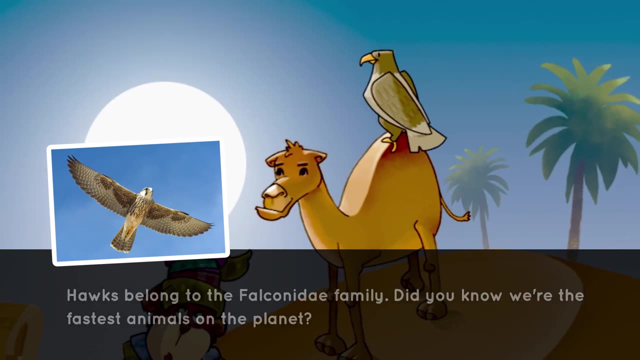 We use it to defend ourselves and protect ourselves from our predators. We live in deserts and sandy areas. Hawks belong to the falconid family. Did you know we're the fastest animals on the planet? Our small size and short, but very wide and pointed wings? 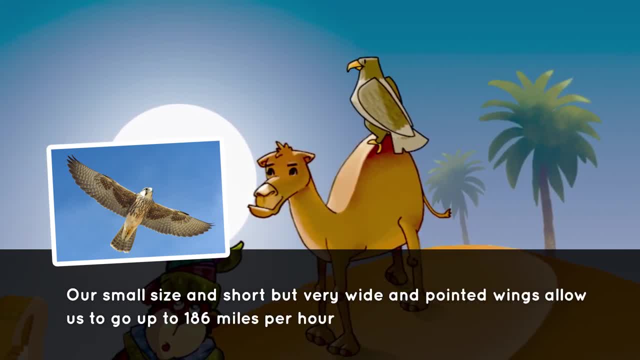 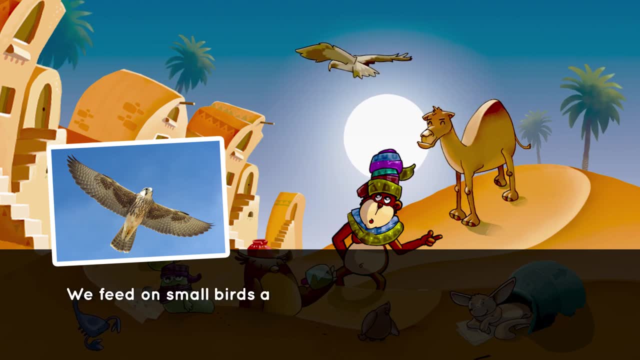 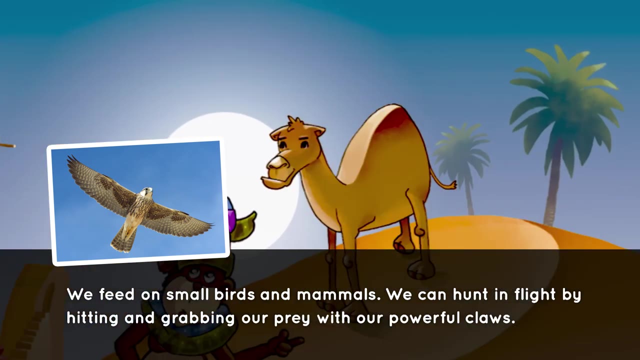 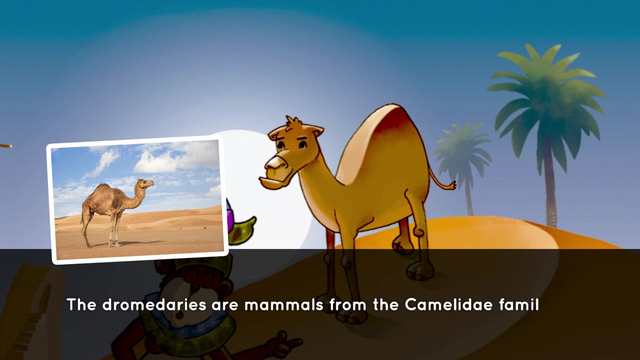 allow us to go up to 180 miles an hour, That's 186 miles per hour. We feed on small birds and mammals. We can hunt in flight by hitting and grabbing our prey with our powerful claws. The dromedaries are mammals from the camelidae family. 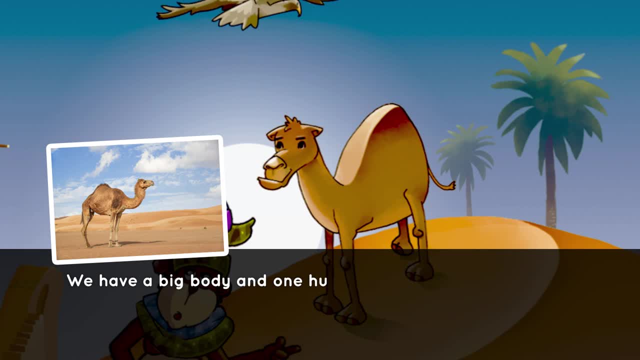 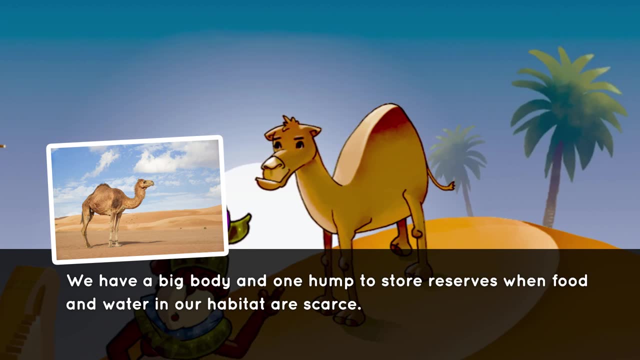 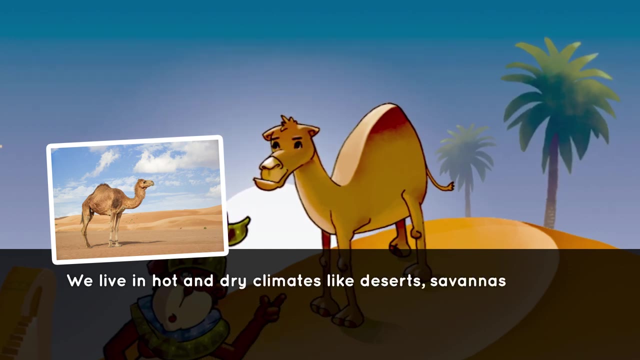 We have a big body and one hump to store reserves when food is needed. Food and water in our habitat are scarce. We live in hot and dry climates like deserts, savannas and grasslands, where it doesn't rain very often.